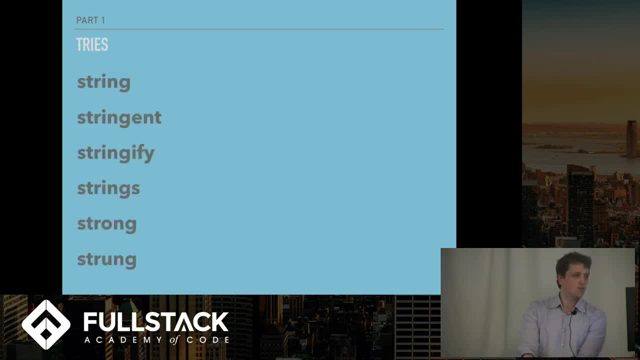 To illustrate this. if we are dealing with many strings, we might have to store strings like this in our array And you'll notice if we have string and stringent and stringify, et cetera in our array, we are repeating ourselves an awful lot. 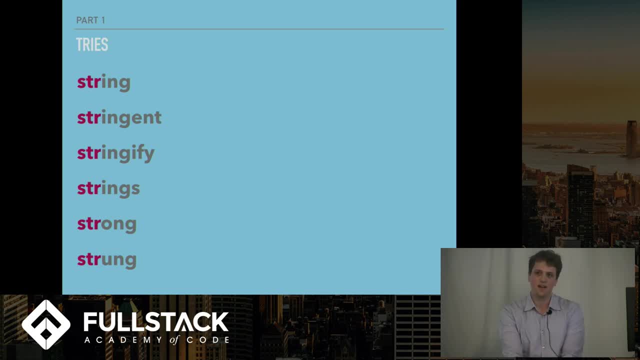 All of these strings share the common prefix st And four of them share the common prefix ing. So what we could do, if we're very clever, is take advantage of the structural similarity among all of these strings and build a tree out of them that would look something like this: 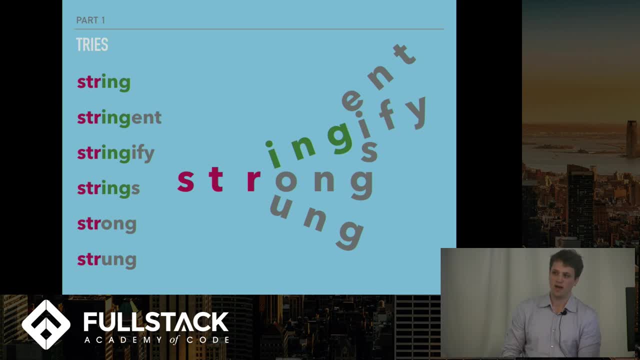 So all of these strings that have a common prefix str grow out of that prefix, and then all of the strings that share the common prefix ing grow out of that one. If we rotate that 90 degrees, we get what's called a try data structure and it looks like this: 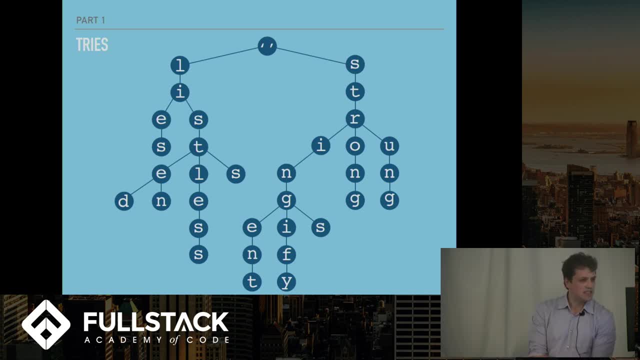 If you read through it, you'll see that we have lies, listen, listed, listless lists and strong, strong, stringify, string strings and stringent, all stored in a tree-like fashion. To illustrate the usefulness of this data structure, I'm just going to walk through a couple methods. 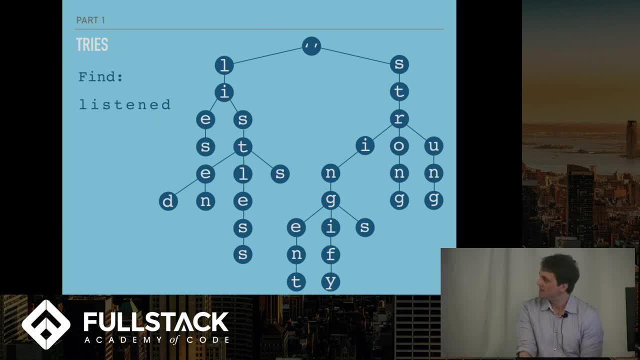 First, the find method. What would we have to do to find listened in this try? Well, all we have to do is iterate through the word we're looking to find and map each character to a path on the try like. so We stop at n and we see that there is a path for the word listen. 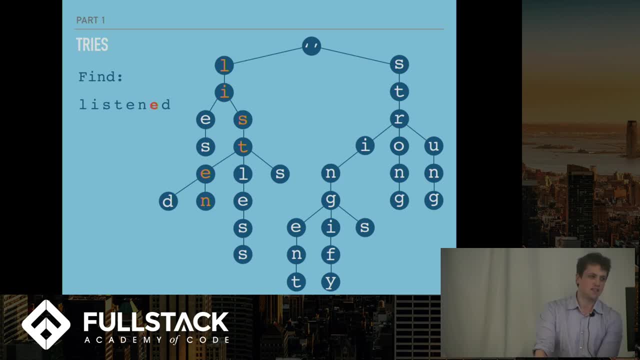 Is there a path for e and d, the last characters of listened? No, there isn't. so we say that the string is not found in this try To insert. all we do is again iterate through the word we want to insert and map each character to a path in the try. 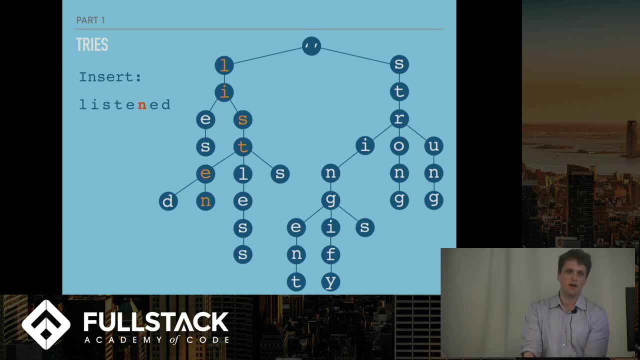 There is a path for listen. there is no path for e and d. so we unlock new nodes, e and d, As you might have surmised. the insertion and find time complexity for a try is O, where n is the length of the string we're looking to insert or to find. 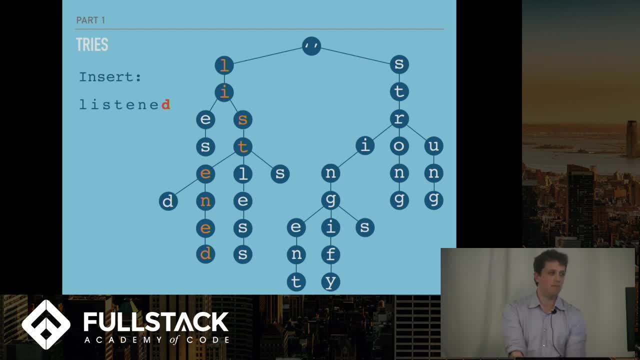 And if we assume that there is a maximum length of the strings- let's say the English language- there's not going to be a word or string more than 25 characters. we can say that insertion and find is actually constant time, So for storing strings they're pretty darn good. 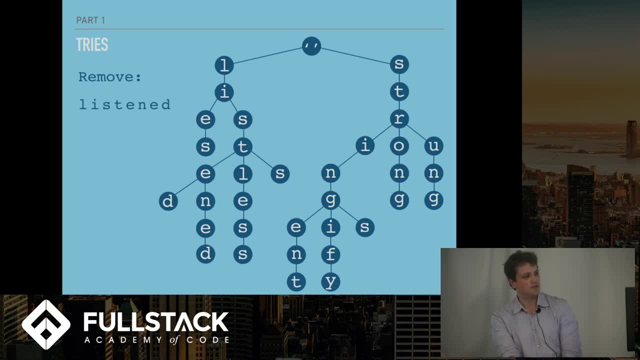 To remove a string from the try, all we have to do is remove the unique suffixes of the string. In this case, the unique suffixes are e and d. So again, we just iterate through the word we wish to remove, map it to a path in the try and then check whether we can safely remove the nodes. 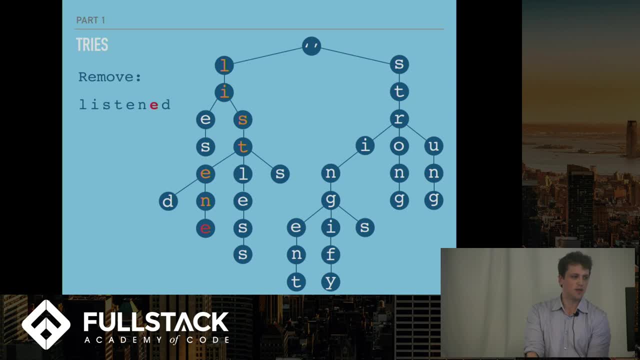 In this case, nothing depends on d, so we can remove it. We go up to e and again see that nothing depends on e. we can remove it. We go up to n and then see that n completes the string listen, so we're not going to remove that from the try. 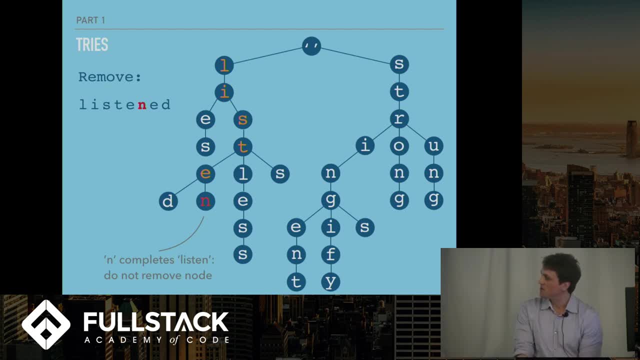 So in this case, to remove the string listen from the try, all we have to do is get rid of two nodes. It's a very quick operation. That ends part one and I want to go to part two. I'm not going to dwell very long on the code. 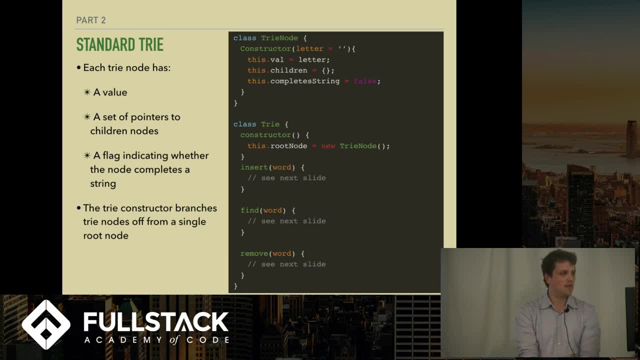 It's a very simple code, and if you want the code, just ask me for it. The implementation of a try is pretty straightforward, at least a simple try. like I showed you, It's a tree structure and so it's going to be implemented like any other try. 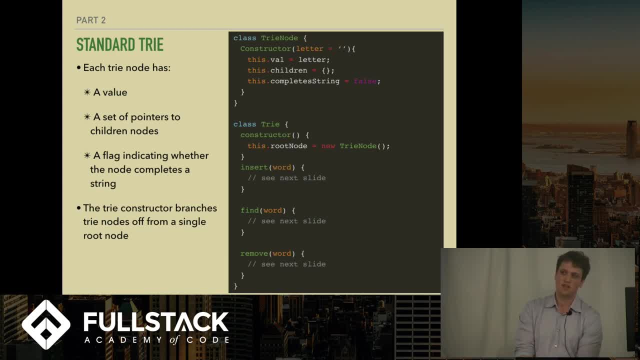 We're going to have a try node constructor function. It's going to take a value and it's going to take a set of pointers to any dependent nodes. That's what thischildren is- And then it's going to take a flag indicating whether the node completes a string in the try or not. 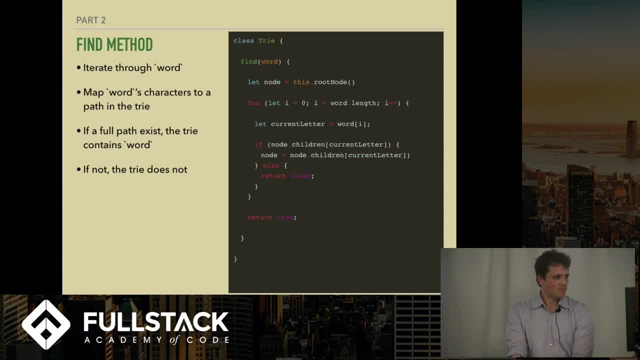 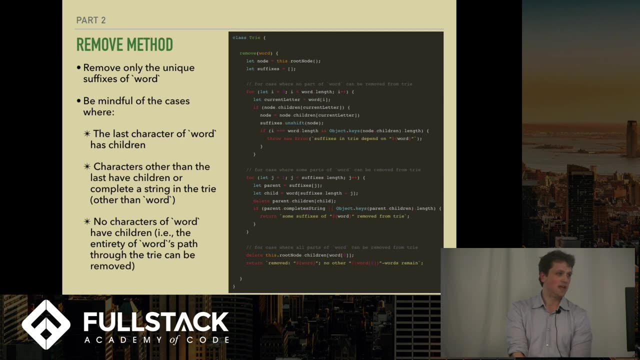 That's what thiscompleteString is. So find is pretty simple. We just iterate through the word. One for-lip will do the trick. Insert looks pretty much the same as find. It's a very simple operation. The only thing that's complicated is the remove method. 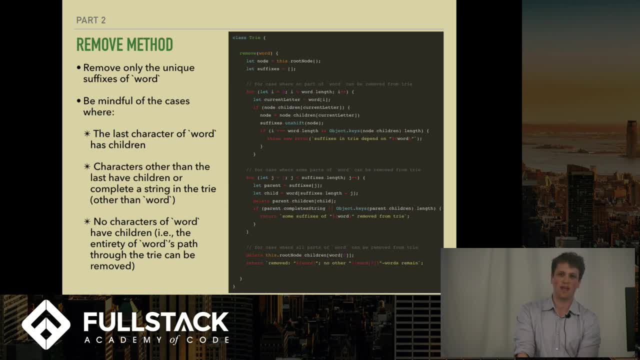 and that's only because there are some funny cases we need to pay attention for, like when we can't remove any character from the string or all characters of the string. But again, it's very simple, You see, just a couple for-lips and it gets the job done. 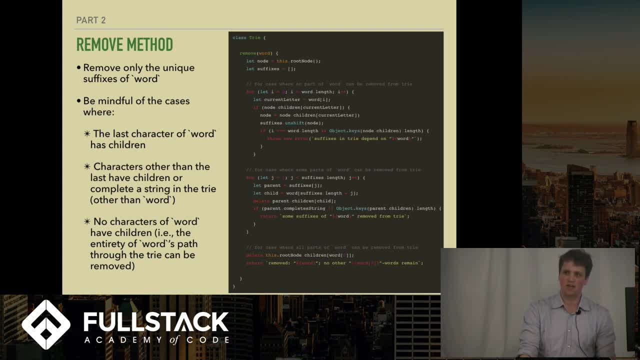 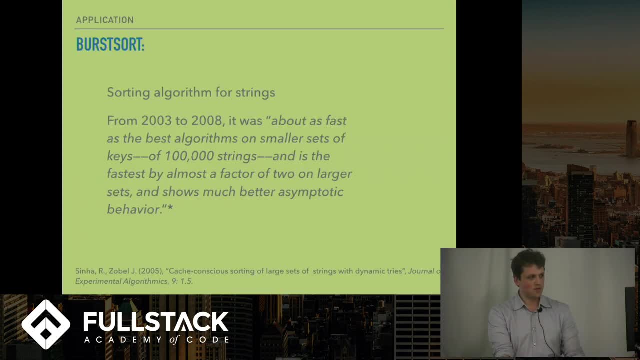 I hope that introduced you well enough to the concept of a try, and I want to go on to something a little advanced called BurstSort. BurstSort is a sorting algorithm and its claim to fame. I'm quoting from the inventors of the BurstSort sorting algorithm. 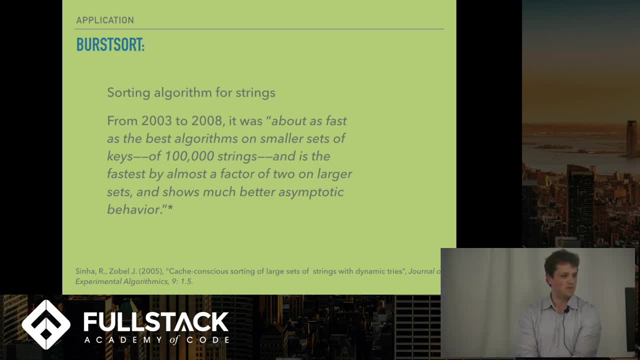 is that it was about as fast as the best algorithms on smaller sets of keys- about 100,000 strings- and is the fastest by almost a factor of two on larger sets, and it shows much better asymptotic behavior than any other algorithm for sorting strings. 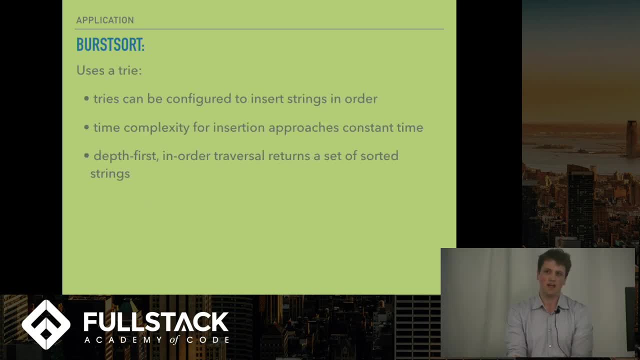 The BurstSort algorithm takes advantage of a try, which is pretty understandable. After all, tries can be configured to store strings already in order. They have an insertion time which approaches constant time, and a depth-first in-order traversal will allow you to pull out strings alphabetically. 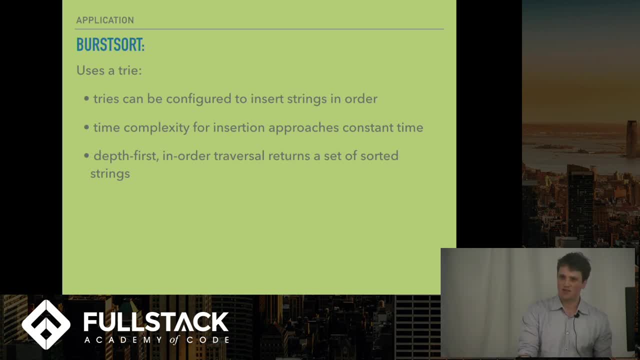 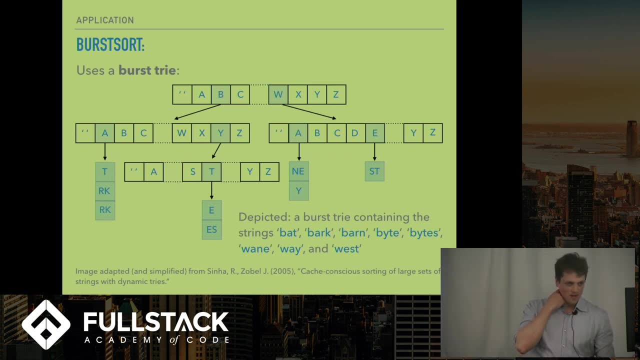 What the BurstSort algorithm uses, though, is not the kind of try that I showed you previously. It uses what's called a burst try, which is depicted here. Here you see the term burst try, which contains the strings bat, bark, barn, bytes, wane, wane and west. 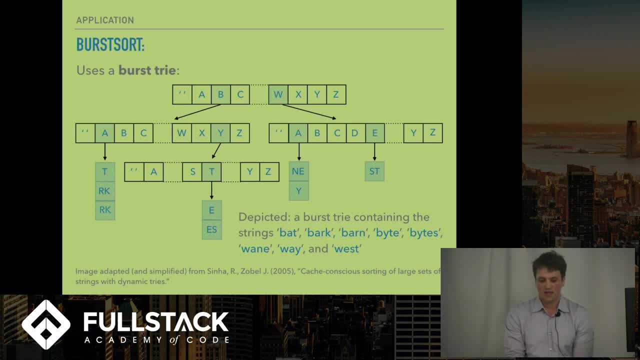 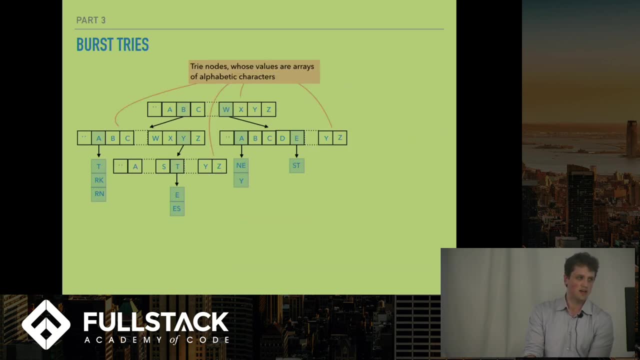 It looks a little intimidating, but it's not all that complicated. There are really only two structural components to this data structure. You have, in the first place, trinodes whose values are arrays of alphabetic characters, and then you have these arrays which are called containers. These arrays have a predetermined size and when they get overloaded they burst into new trinodes and then new containers. The real cleverness of this burst try is that it's division of labor between try structures on the one hand and arrays on the other. 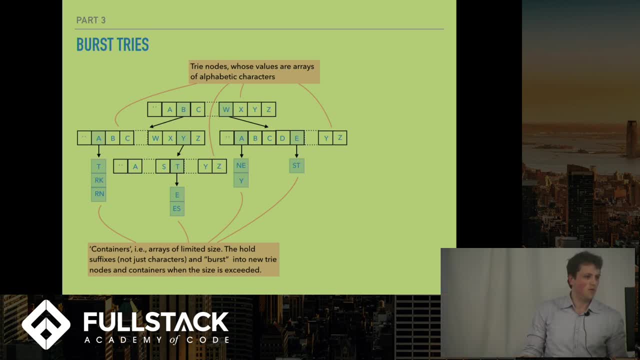 I'm going to point briefly at the screen. I know it looks weird. We wanted to install the word wayward into this try and we were only using tries. to do so, We would have to create seven layers of try structures, each of which is an array of 26 characters, just to store one word. 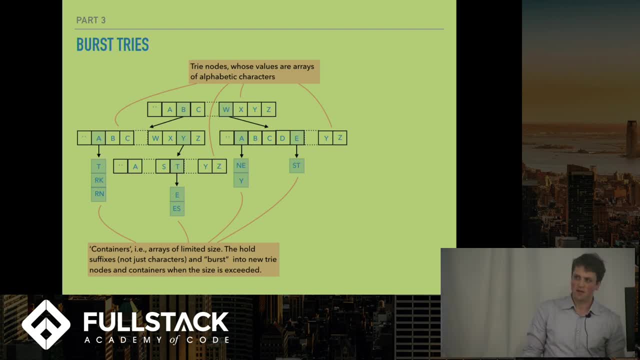 If we wanted to store in addition the term western, we would again have seven trinodes that we'd have to unlock, each of which is an array of 26 characters. These trinodes actually branch out from each other To store these extra long strings like wayward and western. 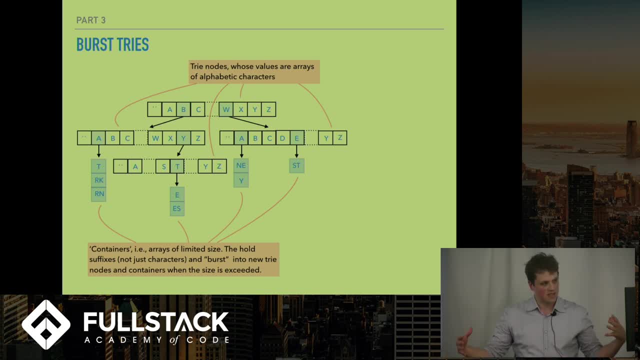 we would have to make it a kind of unruly multiple, like just a large number of trinodes with characters that don't point anywhere and serve any purpose. So searching through them would kind of be complicated and inefficient. So what it does is it takes all of the common prefixes of all these terms. 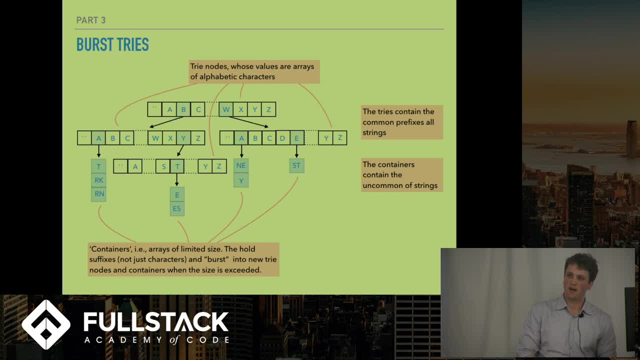 and it puts all of them into tries structures and it takes all the rare, uncommon suffixes and drops them into arrays. Is this? I hope this is kind of clear. I'm getting some. Gabe says it's okay, great, alright.